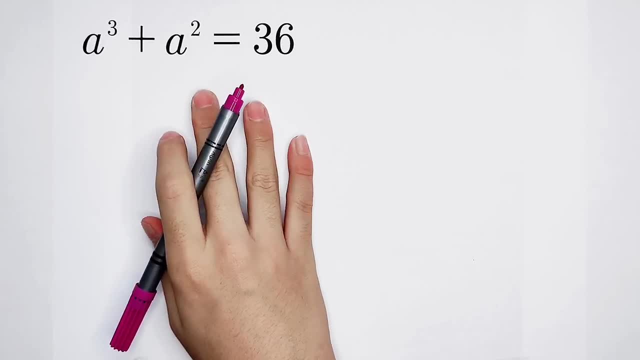 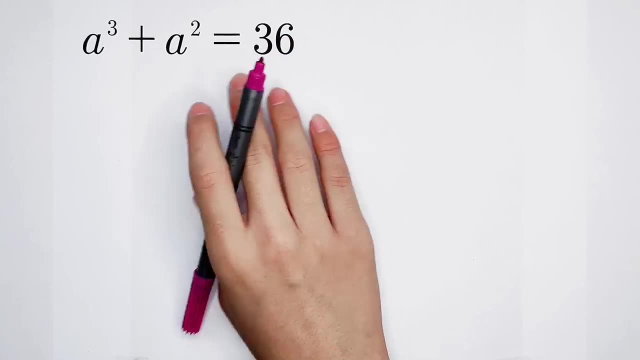 Welcome back to MathWeKnow. Today, we are going to solve this equation. a cubed plus a squared is equal to 36.. It's a common form, isn't it? The term is on the left-hand side and the number is on the right-hand side. 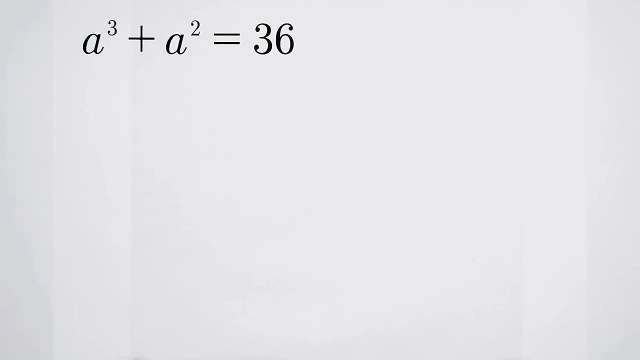 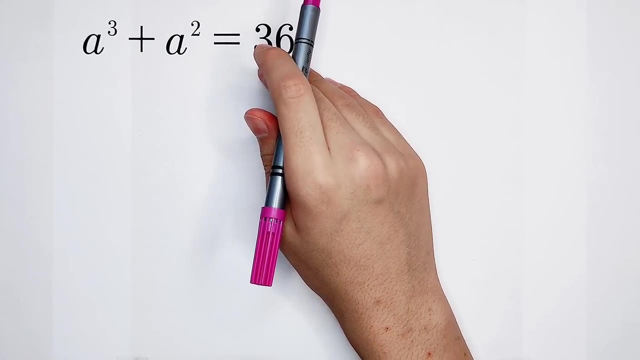 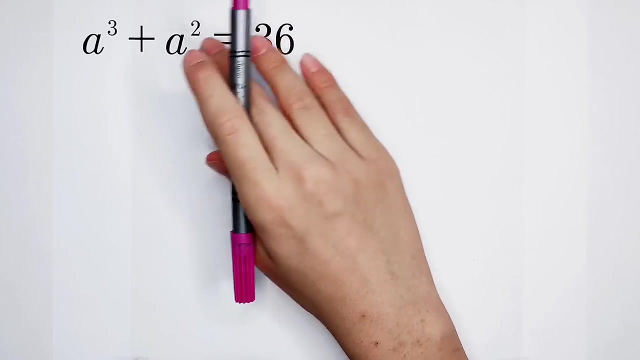 What should we do? How should we deal with it? For dealing with this question, the first step is we should remove this 36 from the right-hand side and move it to the left-hand side. That means I should subtract 36 on the both-hand side. 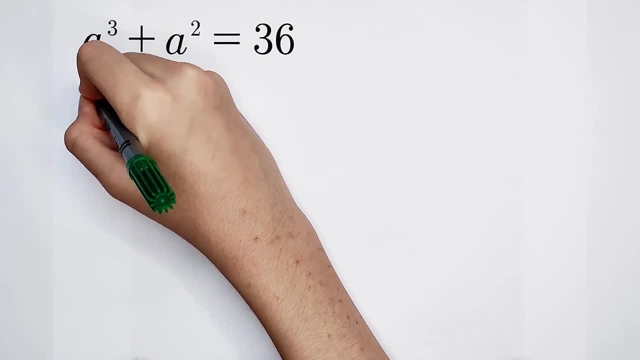 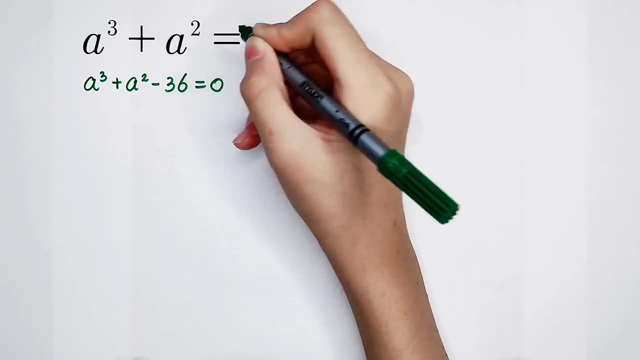 Okay, now have a look at it. a cubed plus a squared minus 36 is equal to 0.. And what should we do? The next step is we should solve this equation. but you see, the largest exponent is 3,, not 2, so it's a little. 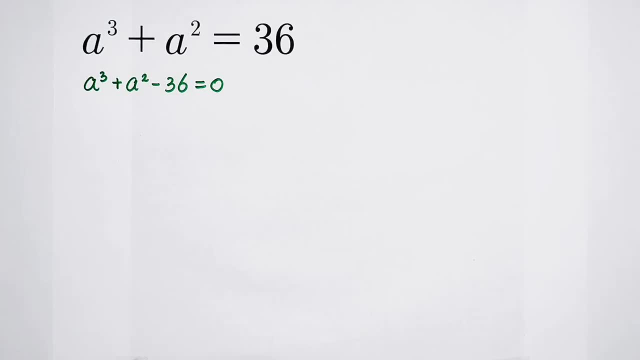 complicated, but I have a wonderful way, Because here appears negative 36,. I think if I can guess a root from this equation and the equation can be hold, that'll be a good news. Okay, then I should guess. Which number should I guess? 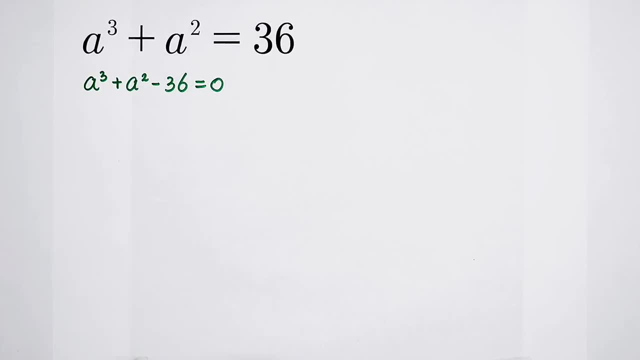 0? No, it doesn't work. 1? Also doesn't work. 2? No. But if you try this number, this lucky number a is equal to 3, then this equation is hold. So a3 is a root from this equation. 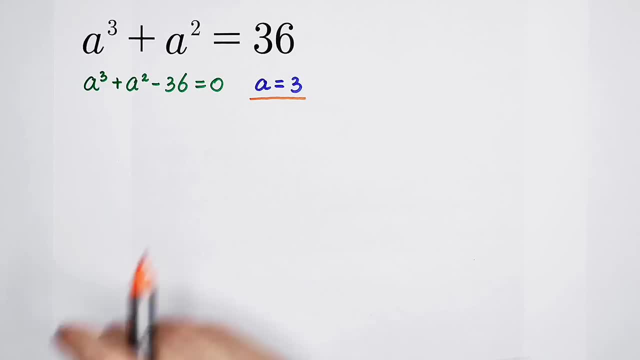 According to the factor's theorem, if a is equal to 3 is one of the roots of our this equation. then we can get: the left-hand side has a factor a minus 3.. Now our work becomes: we should find other roots. 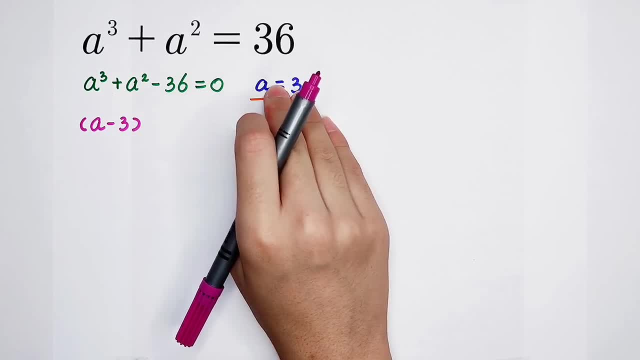 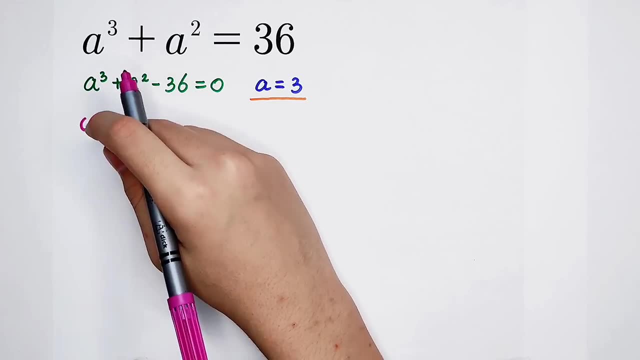 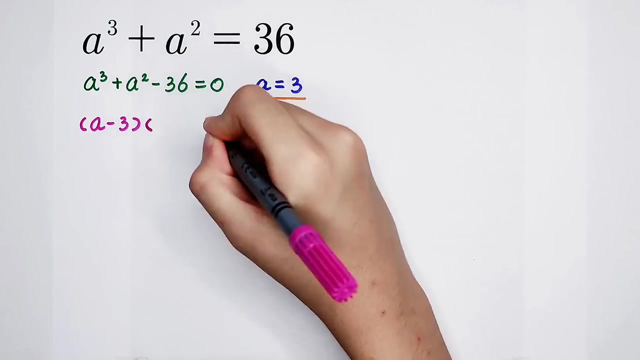 a is 3, is a root of the roots from this equation, And now we have to find other roots. a minus 3 is a factor of the left-hand side, And then we have to find the other factor. So what should we do? 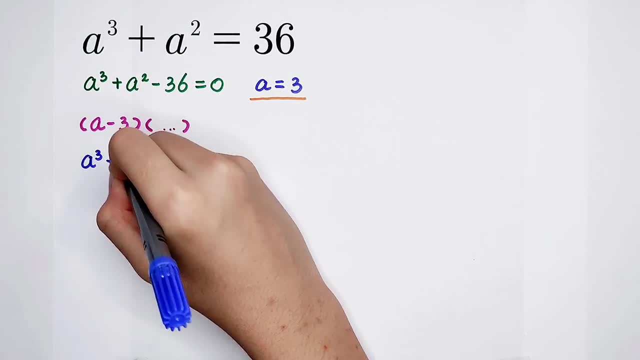 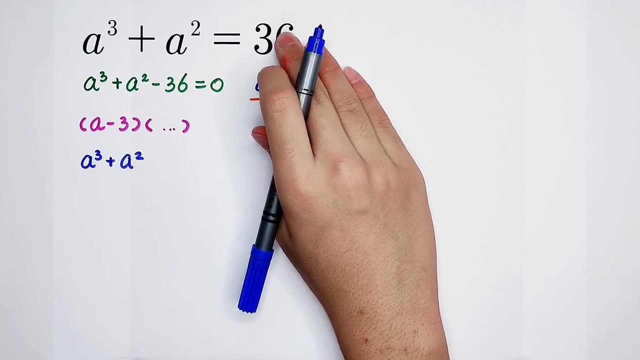 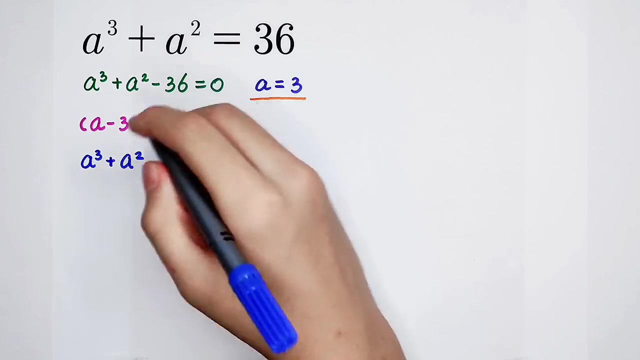 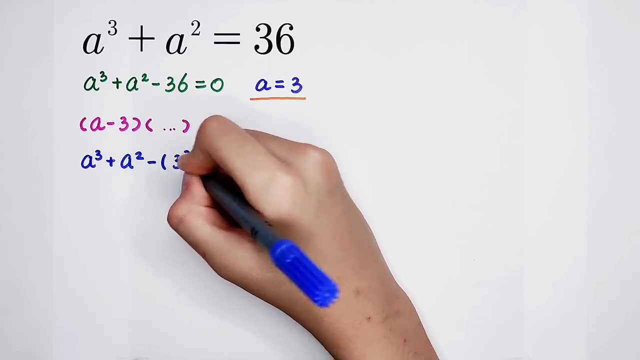 Minus 36, because a is equal to 3, this equation hold. So 3 cubed, then plus 3 squared is equal to 36.. I can write this minus 36 as minus bracket. don't forget: 3 cubed plus 3 squared. 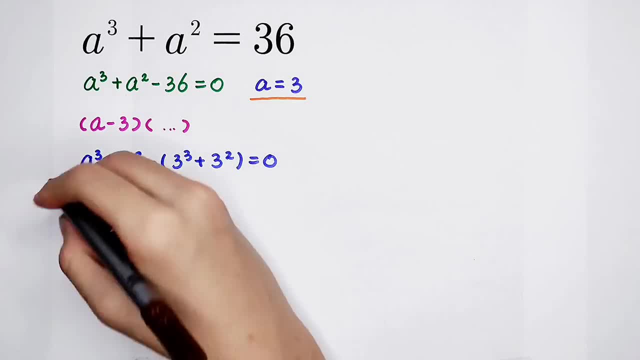 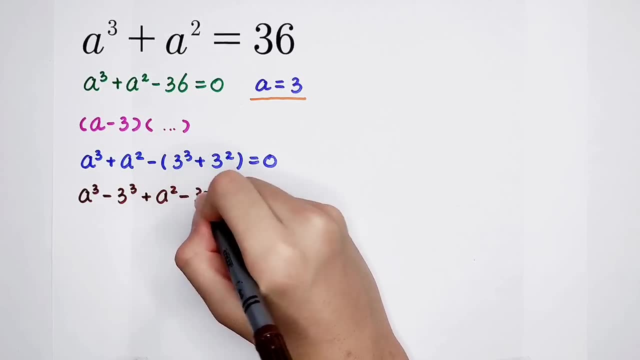 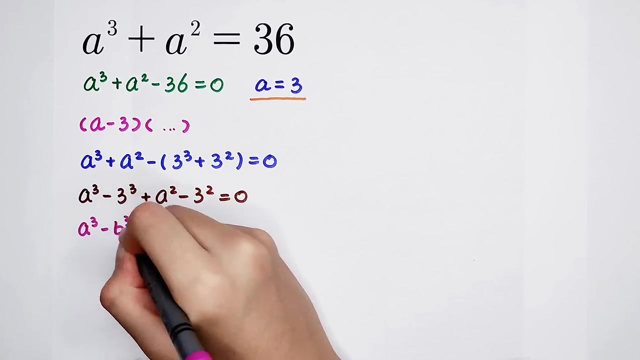 The right-hand side is 0. And then a cubed minus 3 cubed plus a squared minus 3 squared is 0.. Now I need a formula: a cubed minus b cubed is equal to a minus b. then times a squared plus a b, then plus b squared. 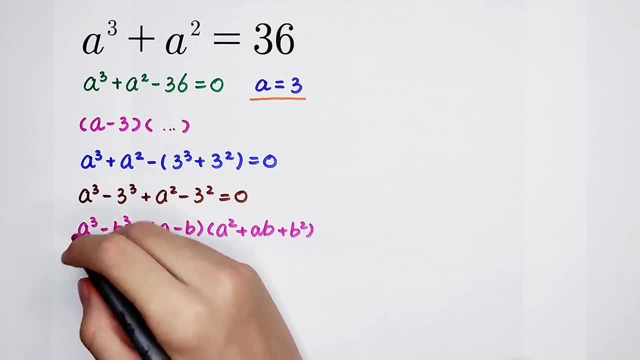 The other formula: a squared minus b. squared is equal to a minus b, and then times a plus b. Okay, these two formulas you can get. What will the left-hand side become? It will become a minus 3, and then times a squared, then plus 3a. 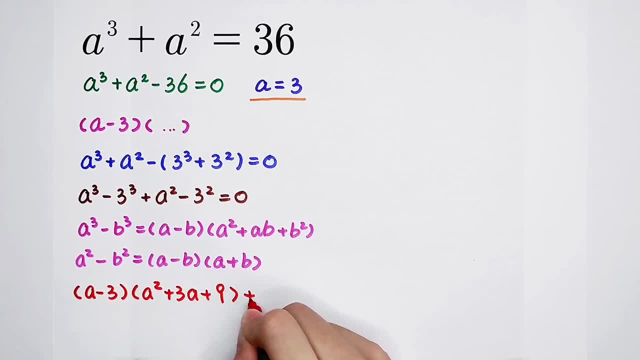 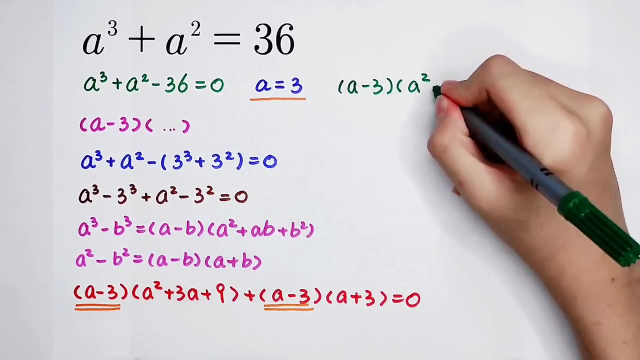 Then plus 9.. And then plus a minus 3, then times a plus 3.. Okay, now have a look at it. the left-hand side, Two factors, So a minus 3 and then times a squared plus 3a, then plus a is plus 4a. 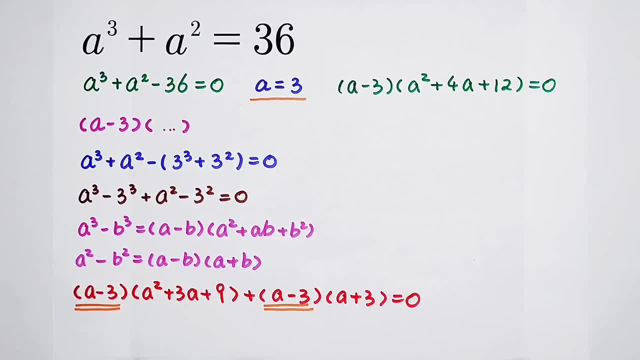 Plus 9, then plus 3 is plus 12 is equal to 0.. And then here we have two cases: The first case and the second case. The first case is a minus 3 is equal to 0. It can be 0.. 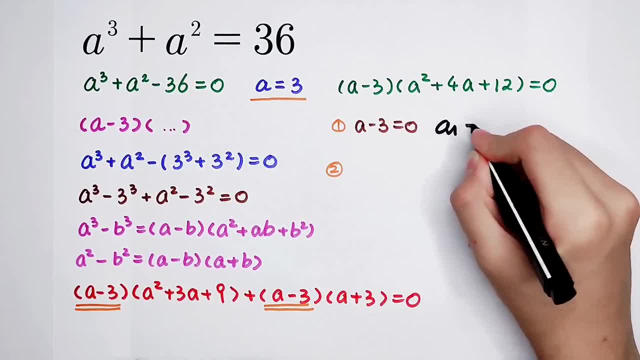 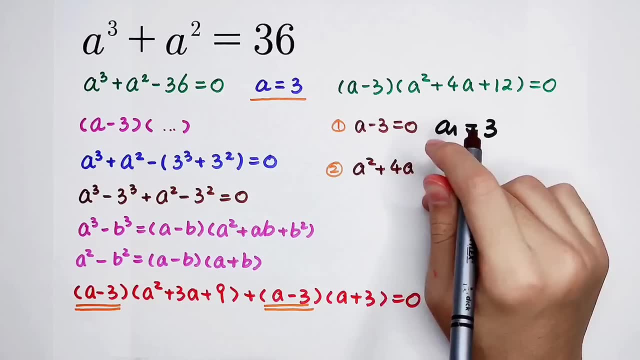 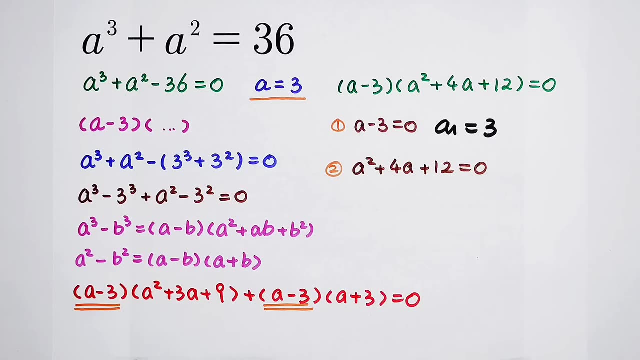 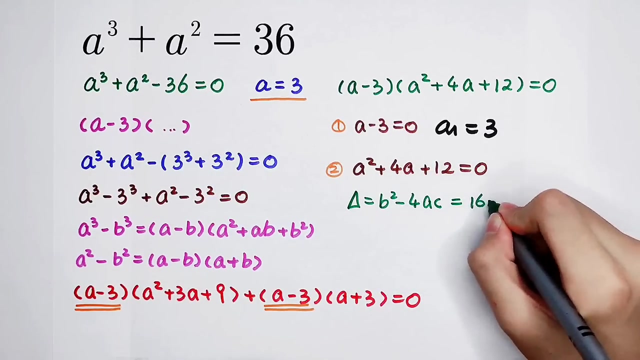 It can also be 0.. Then we can get the first root of our equation: a1 is 3.. The second, a squared, then plus 4a, then plus 12 is equal to 0.. In this case you can get: the delta is b squared minus 4ac is equal to 4, squared is 16, then minus 4, then times a is 1.. 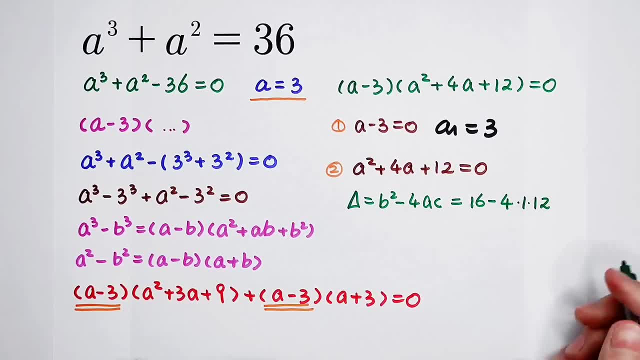 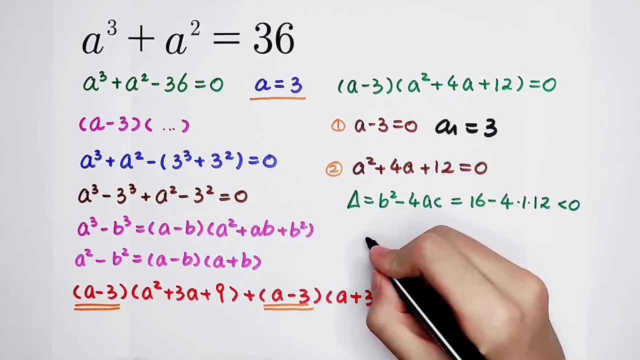 c is 12 is 16, then minus 48. There are no real roots in all this case, So we have only one real root. a is equal to 3. But in the second case- from the second case, Sorry- We can get the other two complex roots. 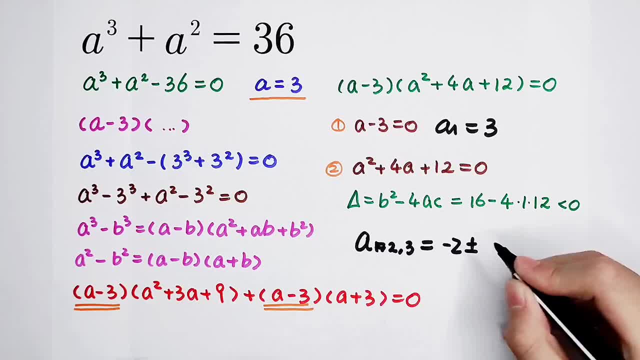 Minus 2 plus or minus 2 times square root, 2 then times i. So there are three roots of our this equation, but only one real root. Did you get it? Don't forget to give me a thumbs up. Subscribe my channel for more videos. Ring the bell And I will see you next time. Bye-bye. Subtitles by the Amaraorg community. 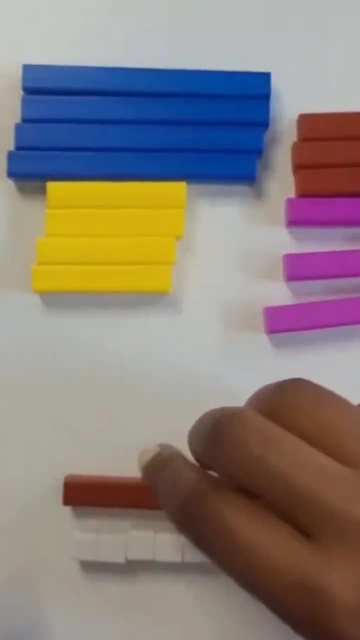 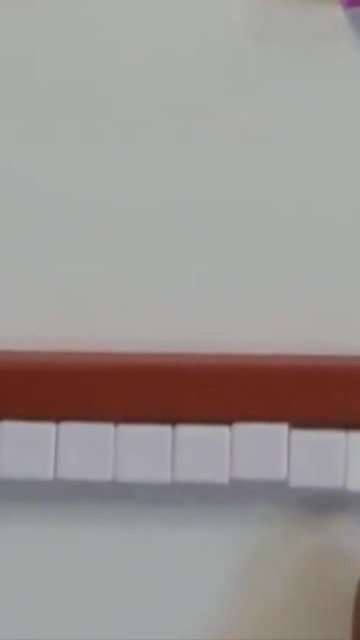 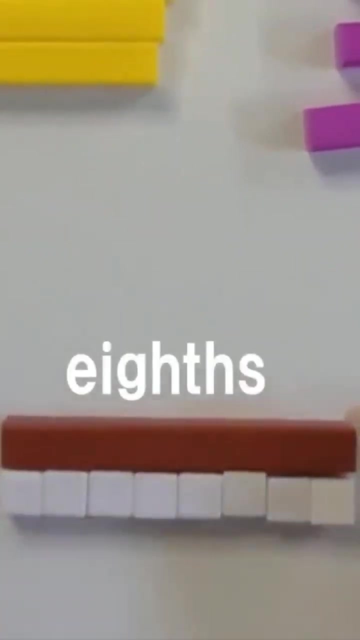 For example, we will use the brown rod as a representation of one whole. Comparing the brown rod to the white rods or units, we are reminded that the brown rod is equivalent to eight white rods or units, So the parts that make up the brown rod can be called eighths, because it takes eight equal. 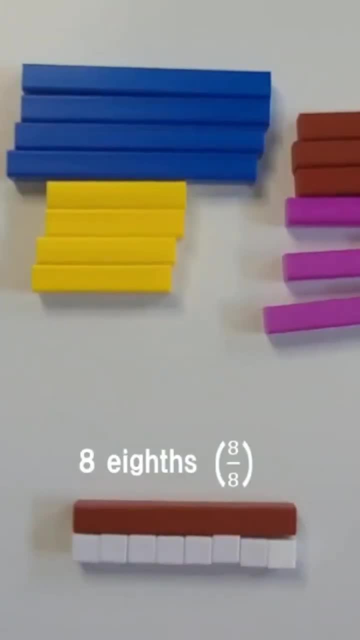 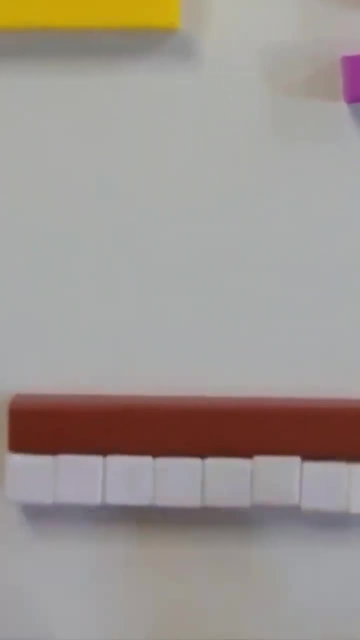 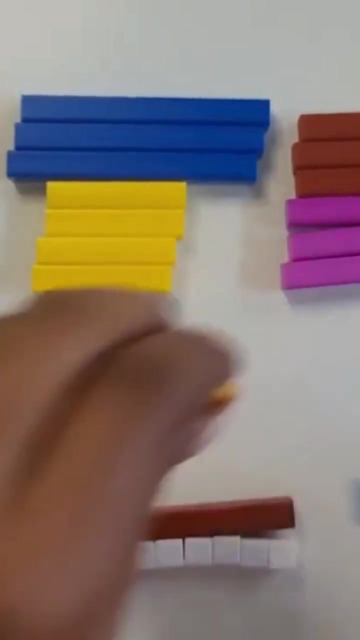 parts to create the whole. Eight eighths is equivalent to one whole. Now we'll find out which other rods or fractions are equivalent to this. one whole or eight eighths? We know that the orange rod will be too long and the blue rod will be too long as well. 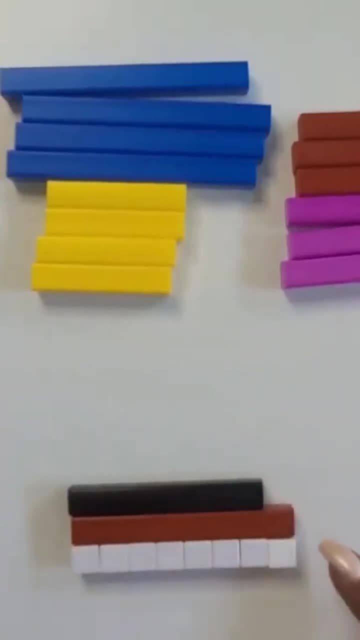 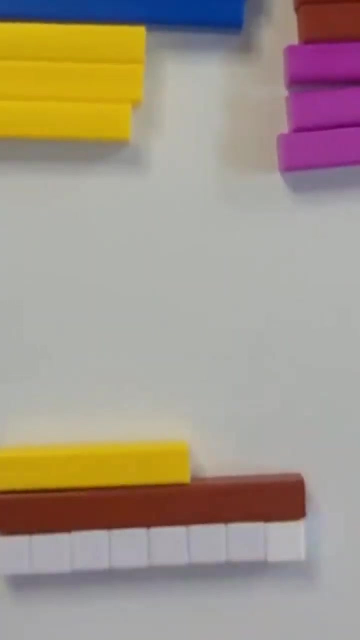 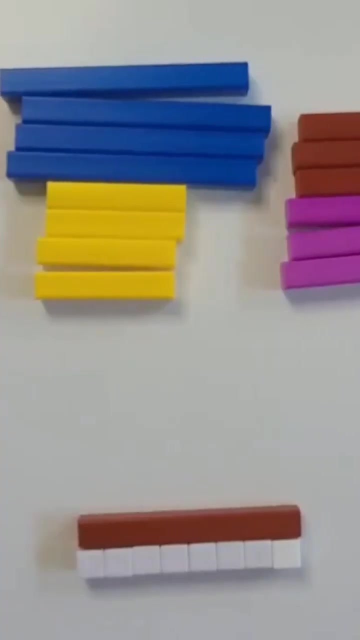 The black rod comes close but is not quite equivalent to this whole, and the dark green rod does not work out either, Unlike in our first example. with this whole the yellow rod is actually greater than one half of the brown rod representing the whole. So now there is just the purple, light green and the red rod.